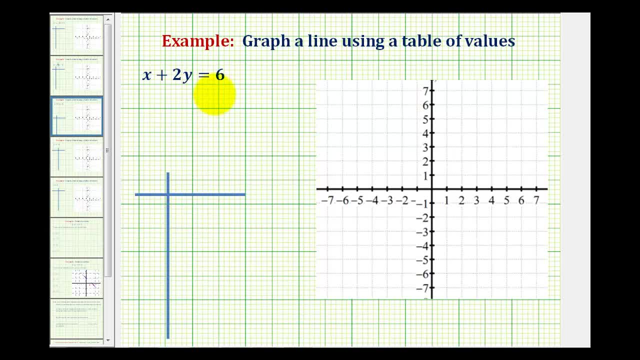 of y, where each x and y value would represent a point on the line. So if we're going to select values of x, sub into this equation and then determine y, it's often helpful to solve the equation for y. So let's start by doing that. 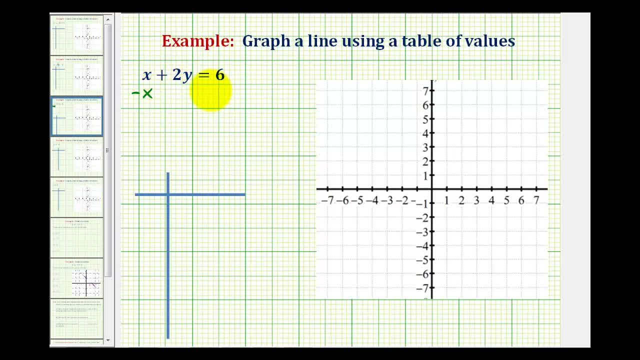 To solve for y, we'd have to subtract x on both sides of the equation. This would be 0. We're left with 2y equals- I'm going to write this as negative x plus 6.. And then the last step to solve for y would be to divide everything by 2.. 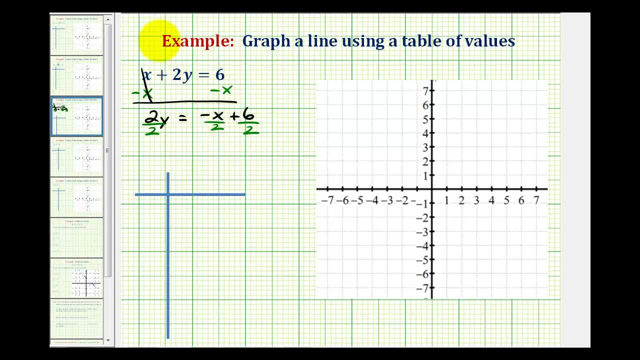 So we'll divide this by 2, this by 2, and this by 2.. So now we'll simplify and the equation we'll use to complete the table is going to be: y equals 2y. Instead of negative x over 2, I'm going write this as negative one half times x. 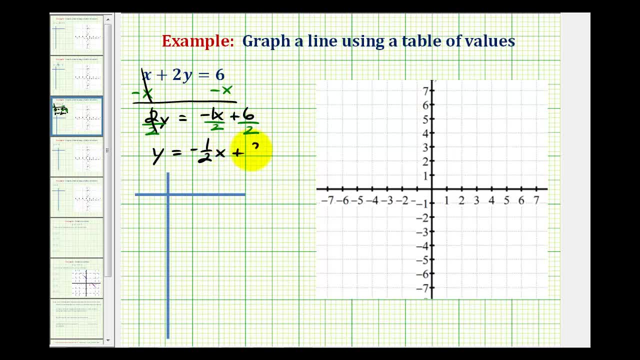 and then 6 divided by 2 is equal to 3.. And now, looking at our table of values, the first column is going to be x and the second column will be y. Now it is easier to graph points when the coordinates are not fractions, so we want to select the values of x. 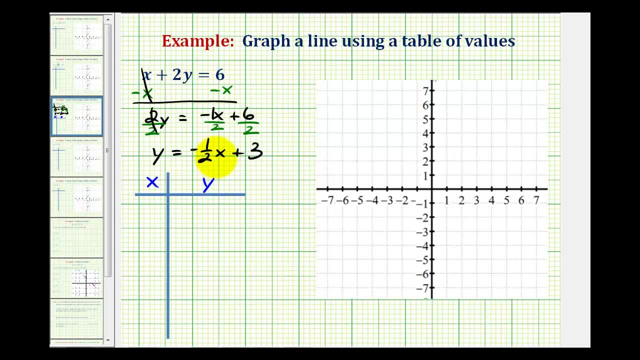 so that when we multiply here, the product will not contain fractions. So we want to select x values. that would be multiples of the denominator or, in this case, multiples of two. So we could select zero, two and four, because these are all multiples of two. 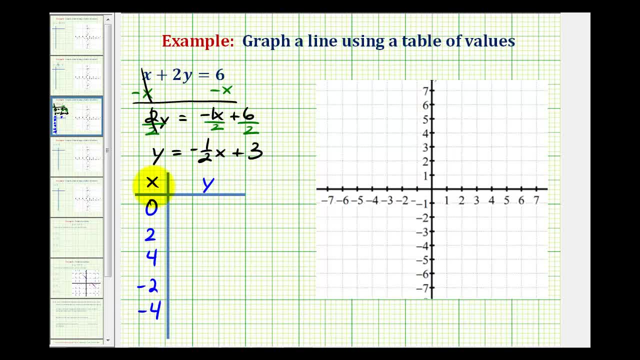 Let's also select negative two and negative four. Now we'll substitute these values into the equation and then determine the corresponding value of y. So when x is zero, we'd have negative 1 1⁄2 times zero plus three, that's going to be equal to three. 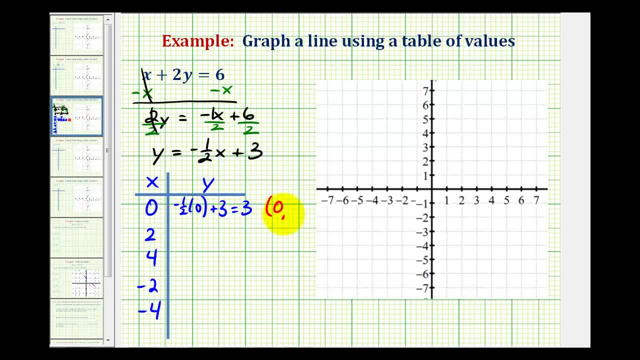 So the point where the x-coordinate is equal to zero and the y-coordinate is three would be a point on the given line. Now we'll replace x with two, so y is equal to negative 1 1⁄2 times two. 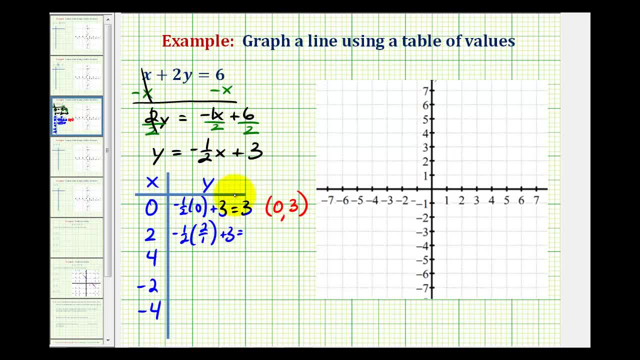 or two over one plus three. Notice how the two simplified a one, so we're left with negative one plus three, that's positive two. So the point with an x-coordinate of two and a y-coordinate of two would be on the given line. 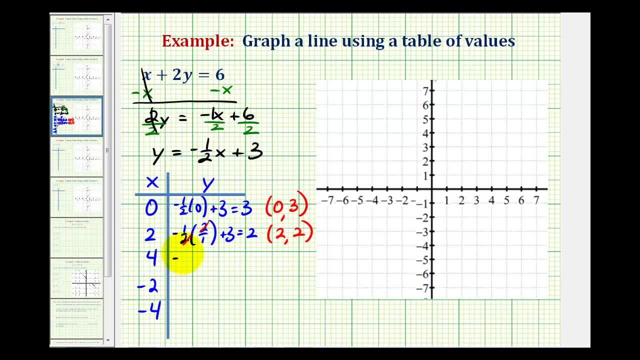 And now we'll substitute four for x. We have negative 1 1⁄2 times four over one plus three. Again, the two and the four simplify. Two simplifies to one, four simplifies to two. So this product would be negative two plus three. 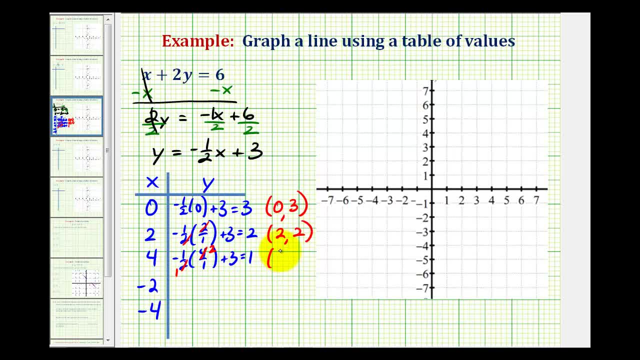 which is one. So the point when the x-coordinate is four and the y-coordinate is one is on the line. Next we have: x equals negative two, so we have negative 1 1⁄2 times negative two over one plus three. 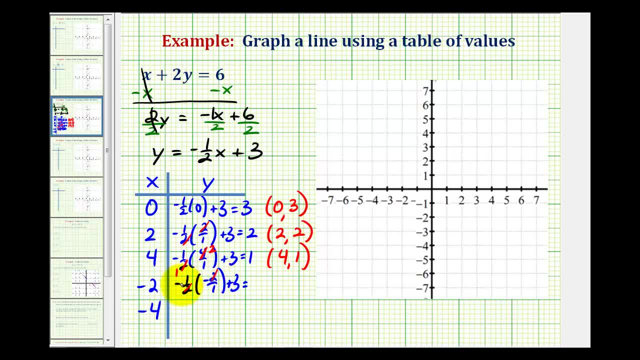 Here's our common factor of two, here and here. So this ends up being negative one times negative one, which is one, plus three, which is four. So the line contains the point where the x-coordinate is negative two and the y-coordinate is four. 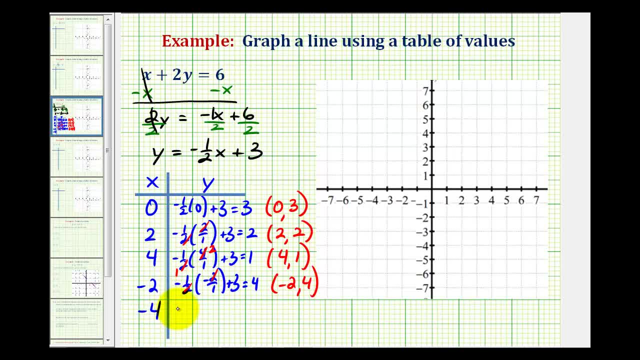 And then for the last x value, we have: x equals negative four. So you have negative 1 1⁄2 times negative four over one plus three. This simplifies again: There's one factor of two and two and two factors of two and four. 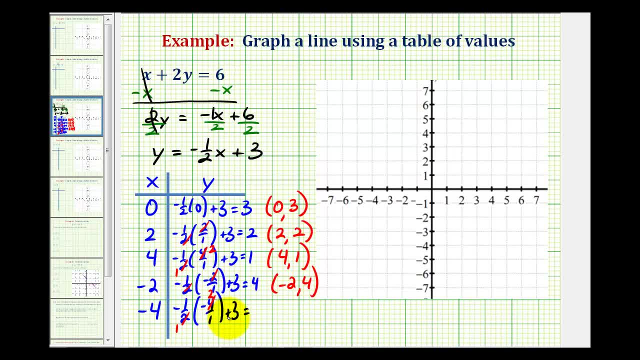 This is negative one times negative. two, that's two plus three, that's five. So the line contains the point with an x-coordinate of negative four and a y-coordinate of five. Let's go ahead and plot these five points to verify they do form a line. 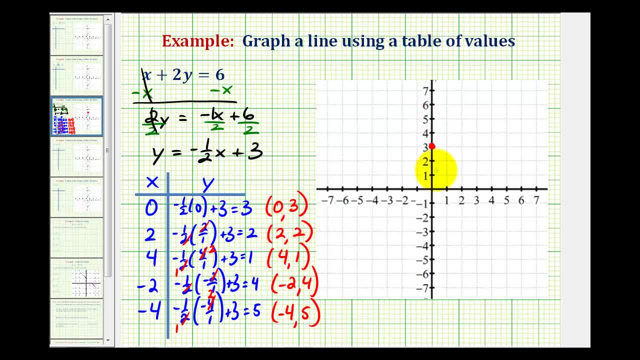 Zero. three would be here: Two, two Right, two up two, Four, one Right, four up one. Negative two, four Left two, up four And negative four, five, Left four and up five. Notice how these five points do form a line. 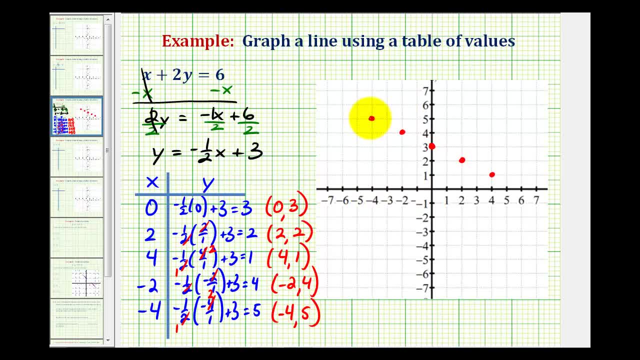 which verifies our work is correct. This would be the graph of our linear equation. Or the equation of this line is: x plus two, y equals six. Or solve for y. we had y equals negative 1 1⁄2 x plus three. 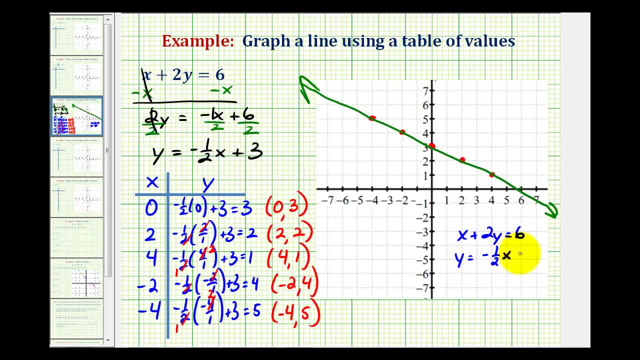 Or solve for y: we had y equals negative 1 1⁄2 x plus three. Or solve for y: we had y equals negative 1 1⁄2 x plus three. These two lines are equivalent, just written in a different form. I hope this was helpful.